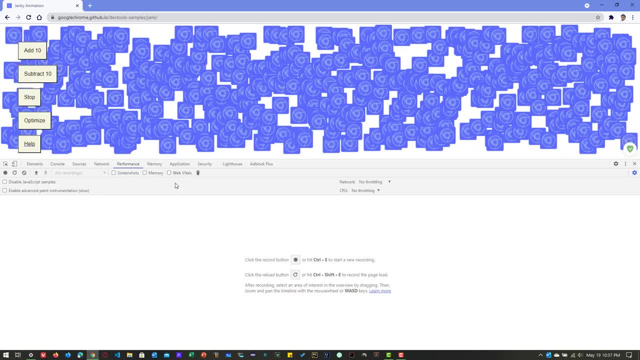 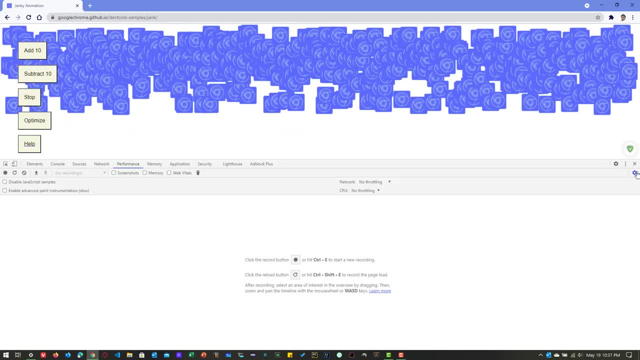 want to check the web vitals, you can do that. And also at the bottom there is a four checkboxes, So this option is available under this capture settings. So if you toggle on, it will display the four checkboxes. If you toggle off, it will go away. 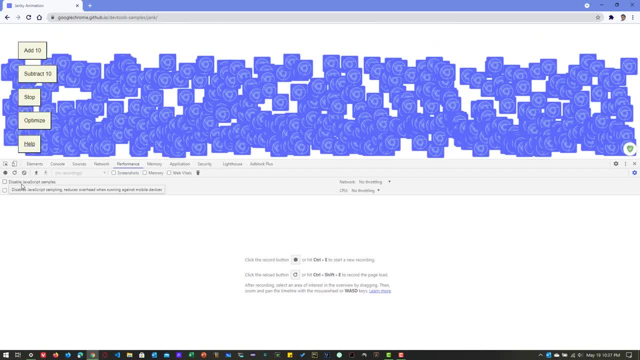 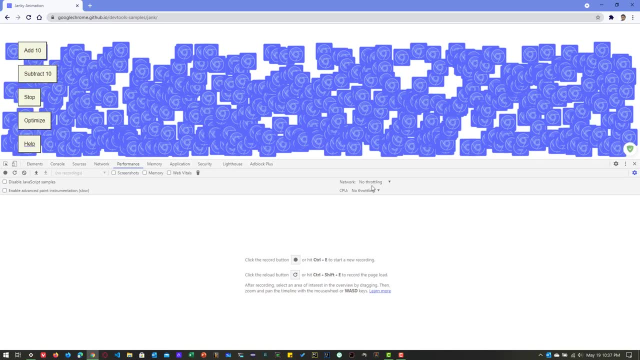 So now here there are four options. First one is the disable JavaScript samples. If you want to disable the JavaScript samples, then you can check this box, And if you want to throttle your application network, you can do that. As I mentioned in the previous video, there are 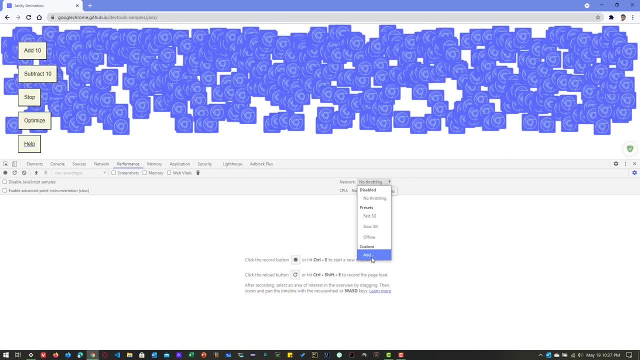 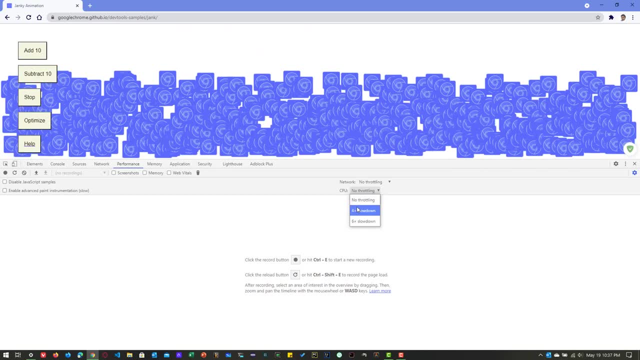 three settings: fast, 3G, slow, 3G, offline. And if you want to add custom profiles, you can add that. And if you want to throttle down your CPU, you can select this option. Basically, it will slow down 4x times and 6x times. 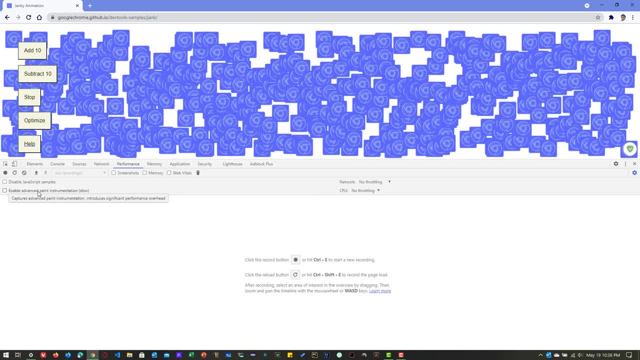 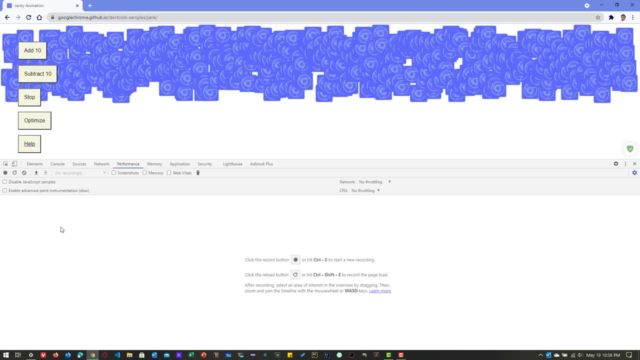 And if you want to display the advanced paint instrumentation, you can check this box, but it will slowly load. It will take more time to display the results, So do not do that unless you know what you're doing. And now we are going to capture this profiling information. 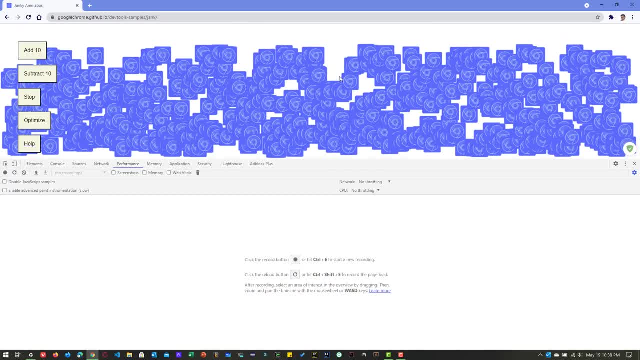 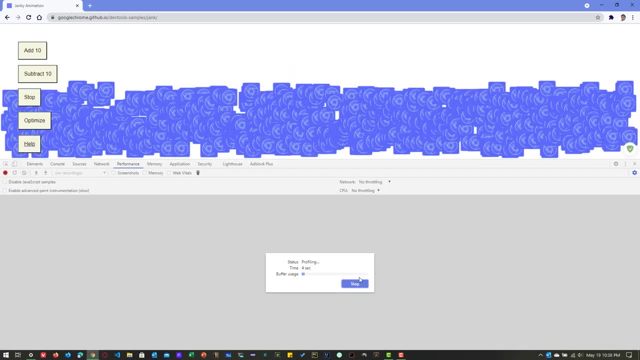 So before that, let me click a couple more times just to make sure that everything is clear. So I'm going to click on this record button and let us leave it for three to five seconds. After it is done, you can just click on the stop button. 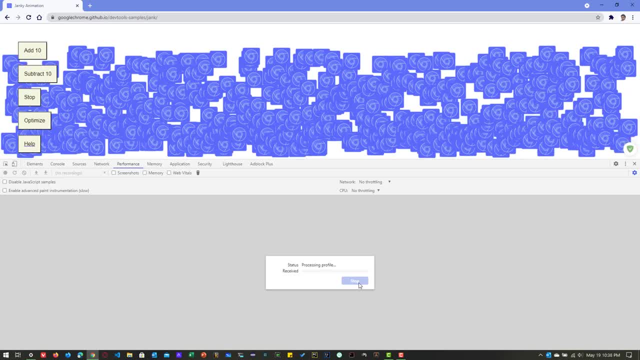 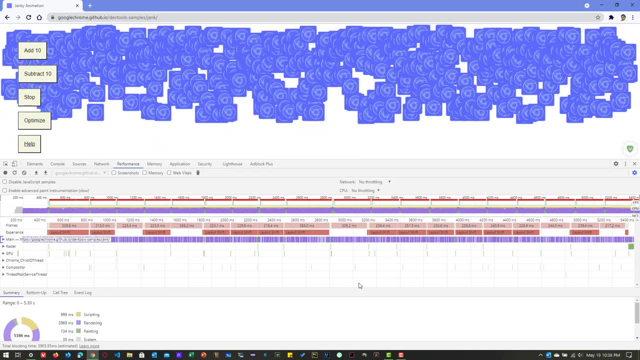 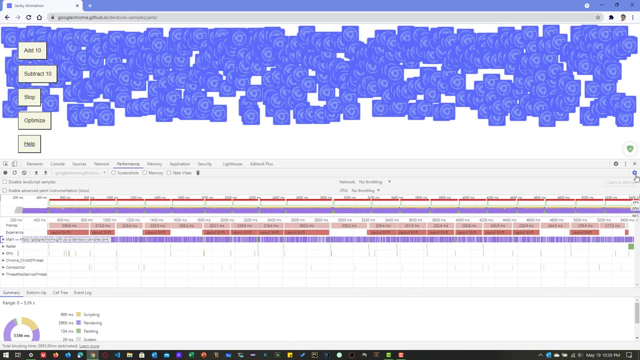 Now it will take some time to display all the details. Basically it will capture everything- frame rates per second, other details- and then it will display flame charts, pie chart, etc. And here you can see it is a time strip, basically very top row. Now let me toggle off this so that 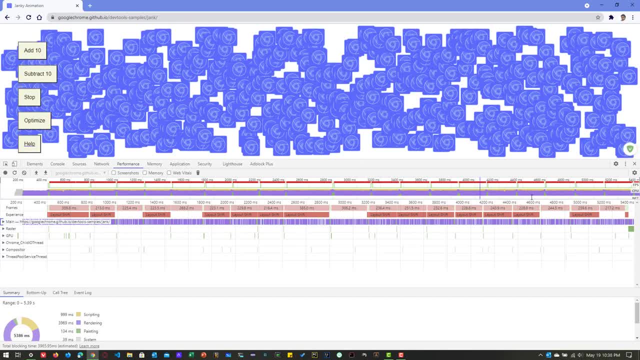 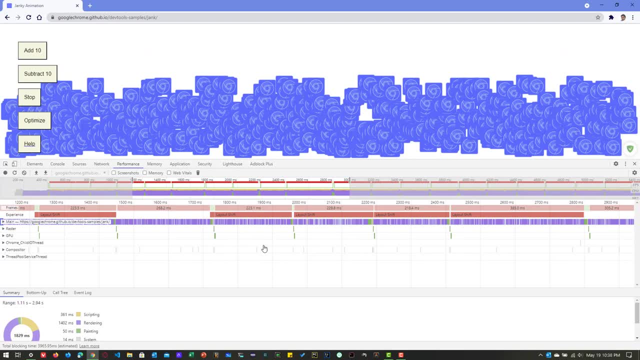 you can see it clearly. Now let me toggle off this so that you can see it clearly. And starting from zero to 5.4 seconds, And here you can just select a particular chunk and then you can just see what's going on, Otherwise you can just double click. 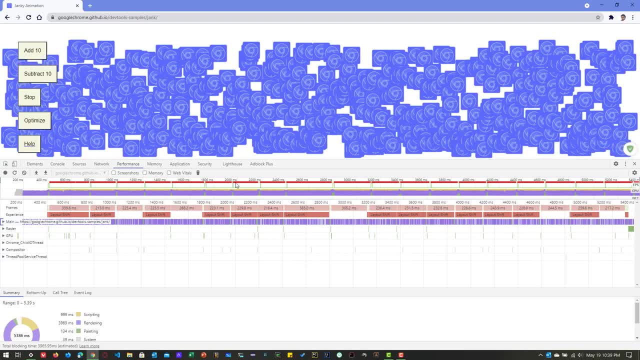 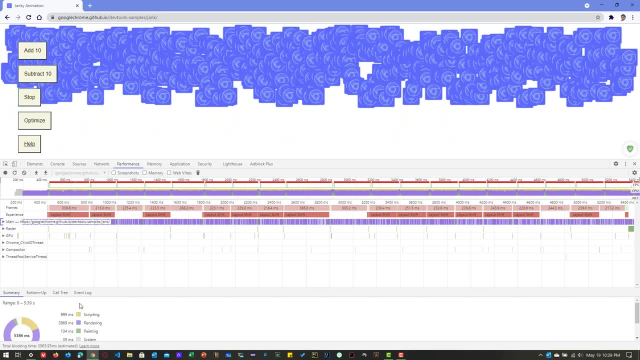 it will select the whole range And whenever you see the red color, basically something is going on, There is some issue, definitely. So that is what the red color means And if you want to see the color coding, you can see the summary. Basically the purple. 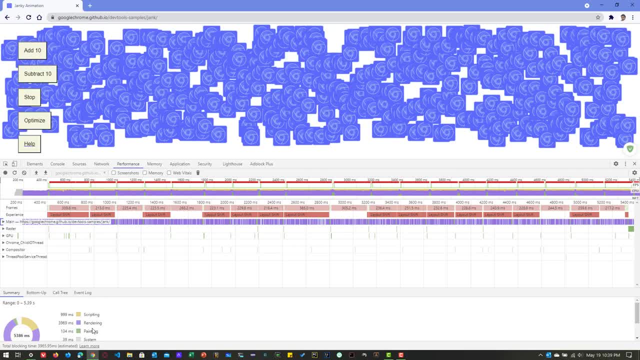 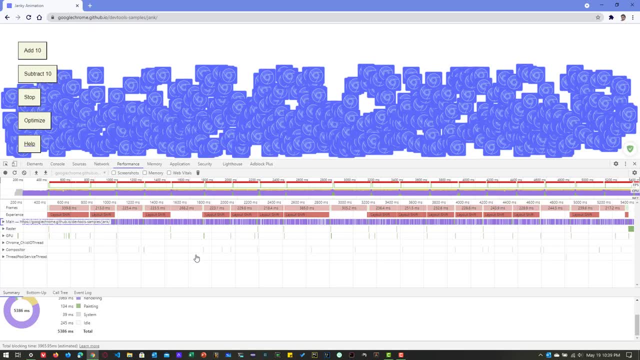 or violet color, it says rendering, and yellow means scripting, and green means painting. Go only you can see the other details. So now let us go with the direct ones. basically, There is what the issue is. So we have to focus on the regular ones, And here, if you just 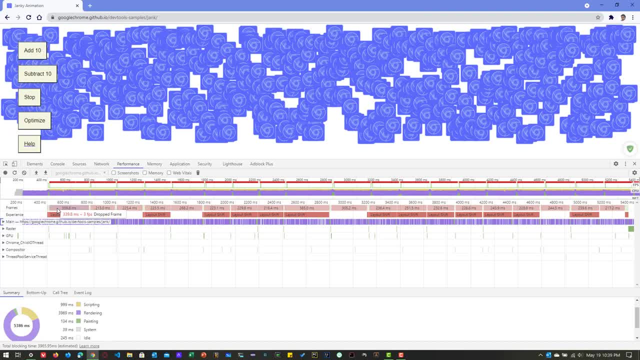 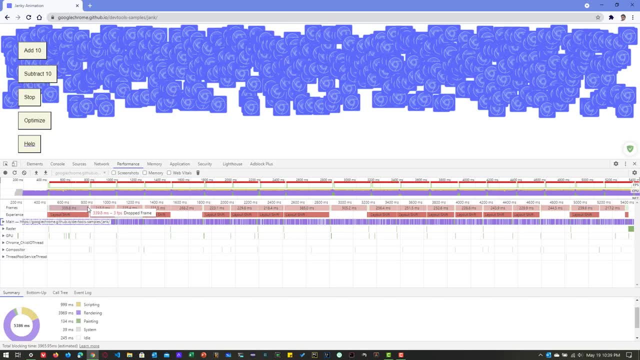 your mouse over the frames you can see drop the frame Some, meaning there is some loss in the frames in the application. that is why it does display in the red color. But if you just hold your mouse over the green color ones you can see there is an increase in the frame per second. 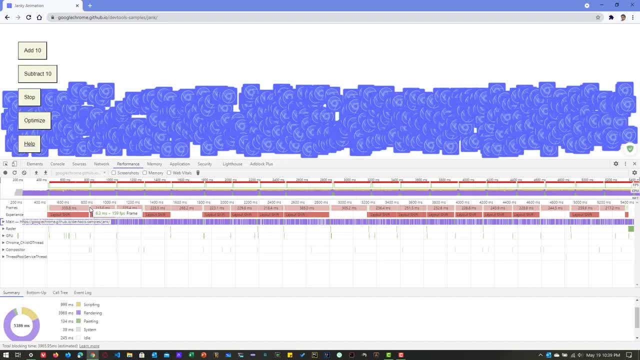 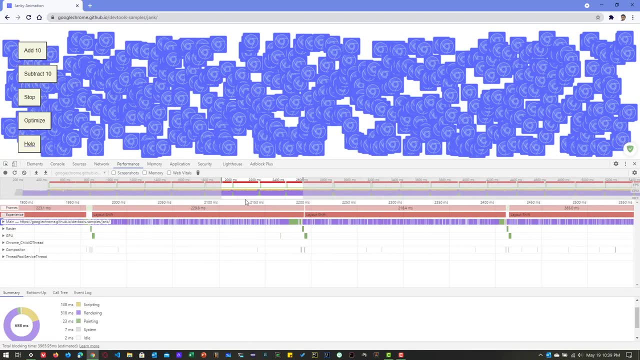 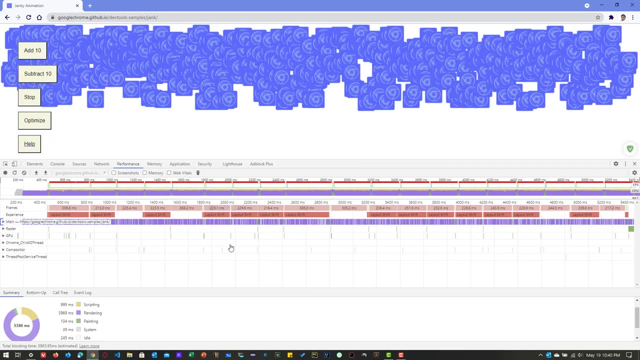 the green ones means it is a good at the time, and if it is a red one there is something going on and if you just- again, if you drill down- zoom in, you can see the details more clearly. basically, and if you just zoom out, you can see the whole chunk. and now i'm going to expand this main. 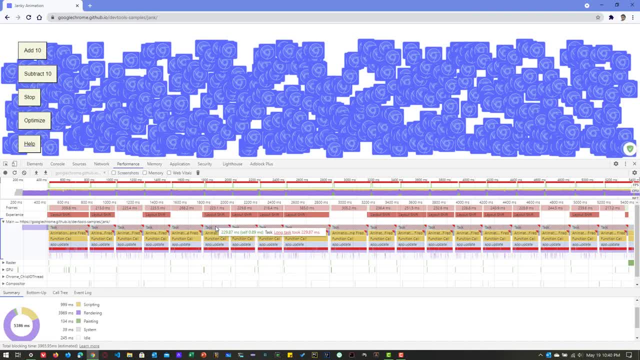 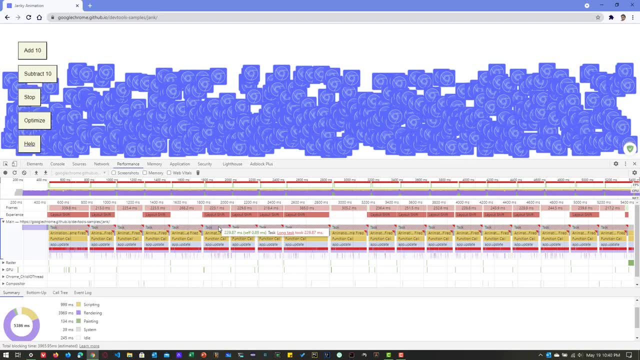 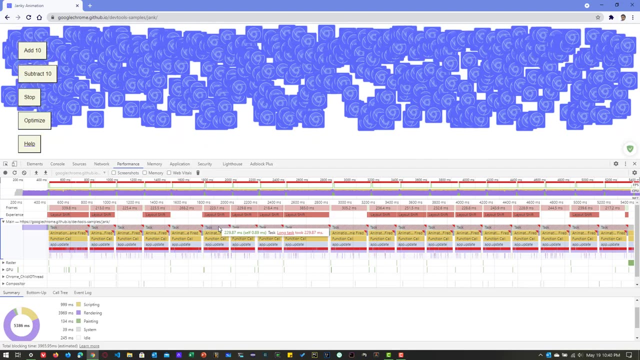 section here and here you can see there are other couple more red colors basically, and if you just hover your mouse over the task you can see there are two things. one is the green one, which is 229 milliseconds, and the task long task basically. so it is taking long time to finish the. 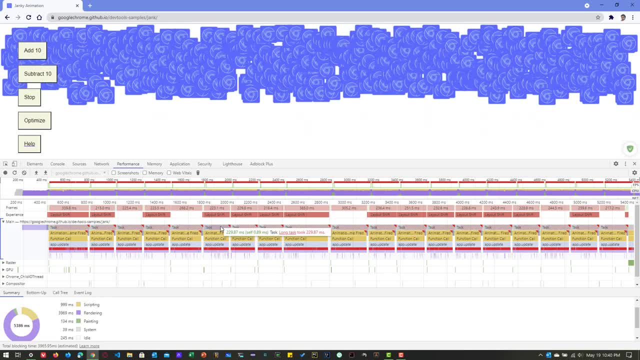 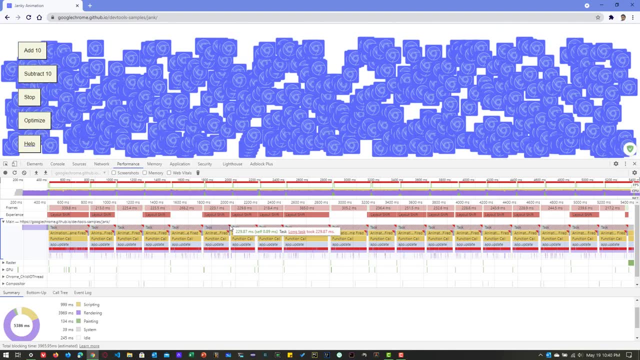 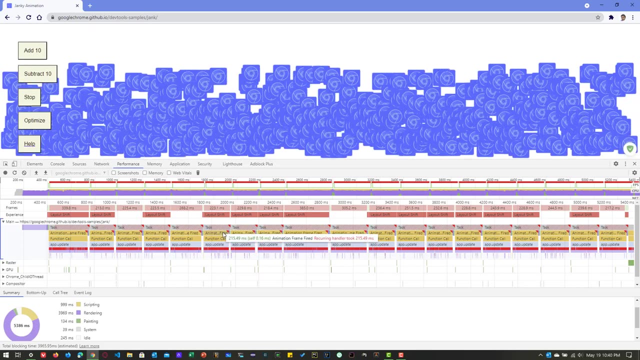 particular task and at the top right of this chunk you can see there is a small rectangle. basically so, whenever you see the small rectangle the top right, so that is the frame which is causing some issue, basically so, here you can see again the animated frame fired, which 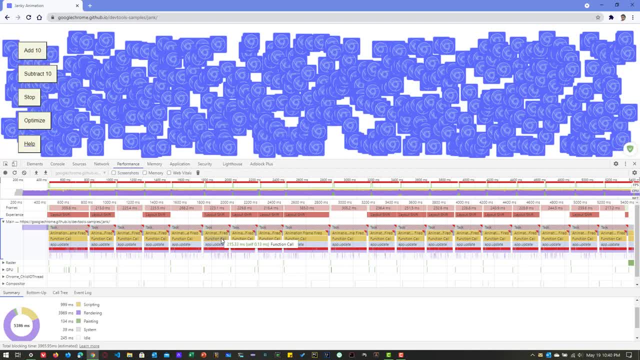 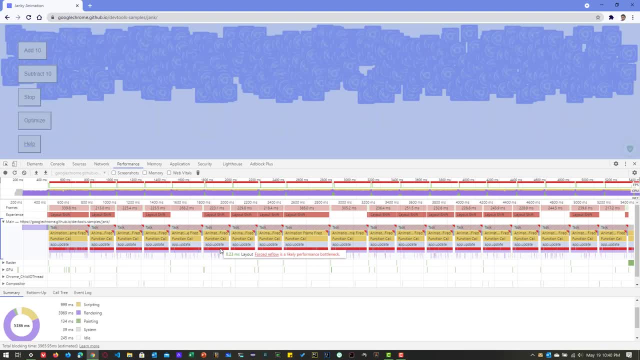 took the long time and if you just scroll down now you can see the function call and the appupdate and again there is a forced reflow, likely a performance bottleneck. so here you can see it is clearly displaying something bad is going on. so how do you pinpoint which line of code? 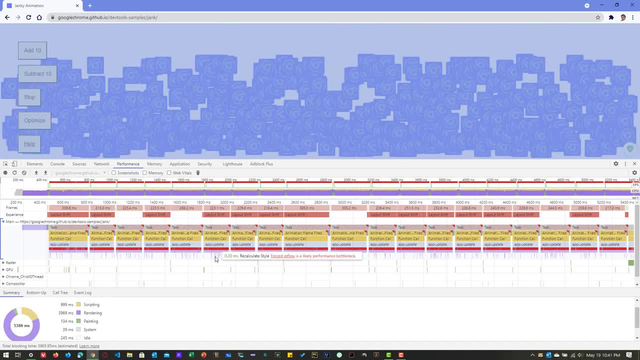 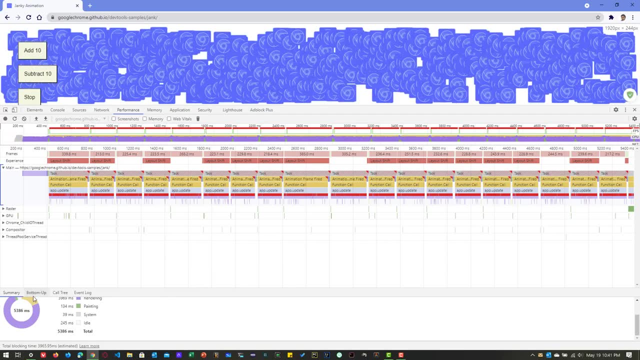 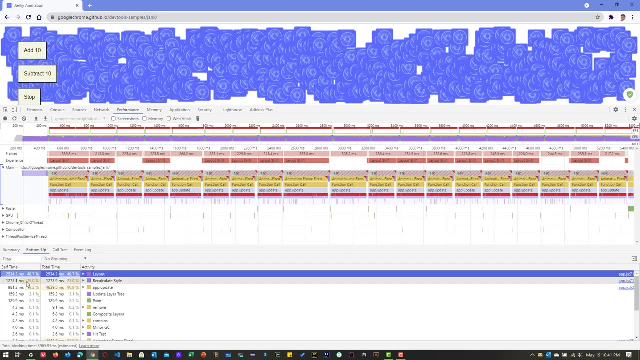 which is causing the issue. so to identify that, if you just scroll down to the summary part here- so let me just expand- and in the summary you can see the pie chart and if you click on the bottom up you can see the table view and the call tree again, 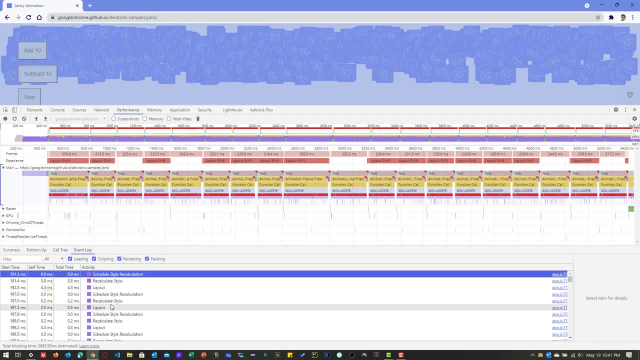 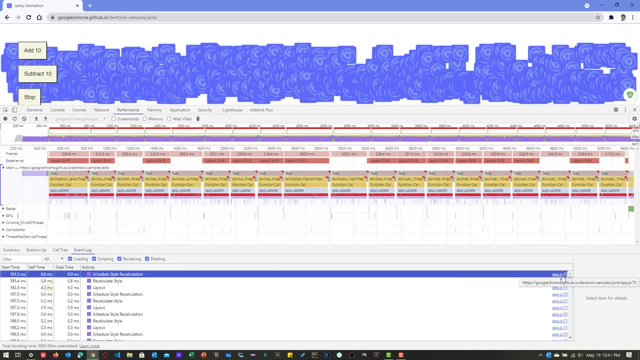 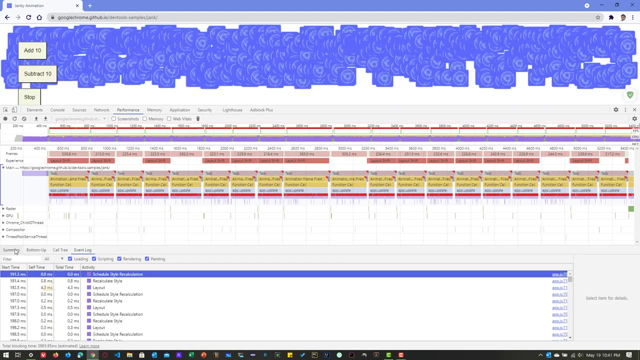 it will display the activity and the event log. it will display the detailed events and the detailed events. you can see at the top right there is a line which is pinpointing appjs. this is the file which is causing this issue and the line number is 70. so this information should be available over. 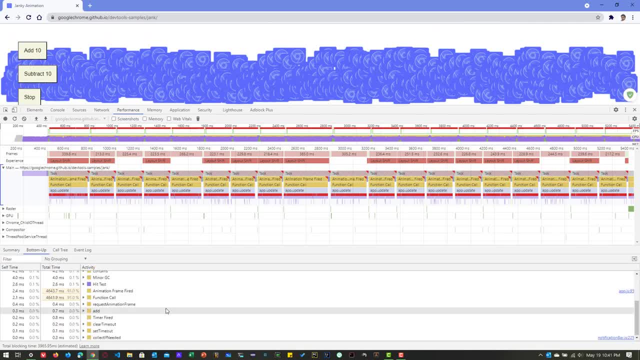 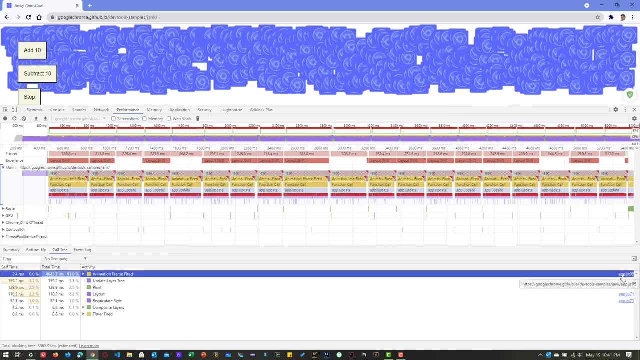 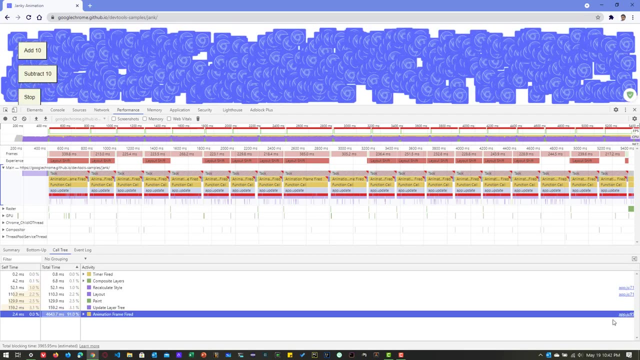 here as well. let me click on this. yeah, here also it is available. you can see the right side and in call tree also it should be available here on the right side and you can sort by the time, total time etc. so here you can see the animation frame fired appjs, line number 95.. so there are a couple of lines where 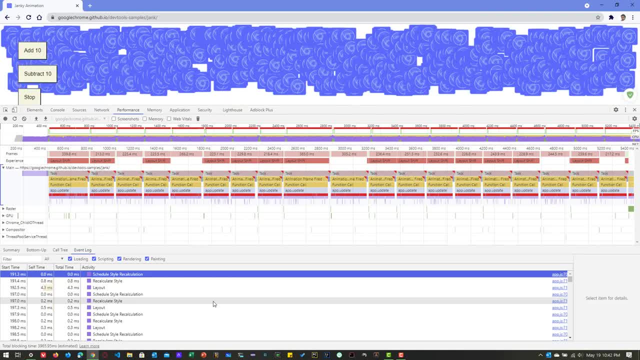 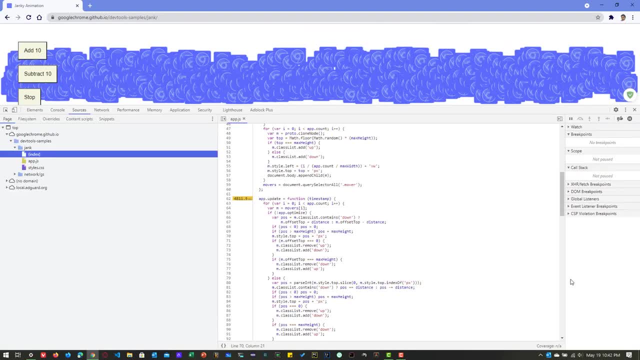 you can focus for the performance optimization. and if you want to go to the particular line, what you can do, you can just right click and you can click on the reveal in sources panel. so you're So, if you click on reveal in sources panel, you can see the line, exact line, number, line. 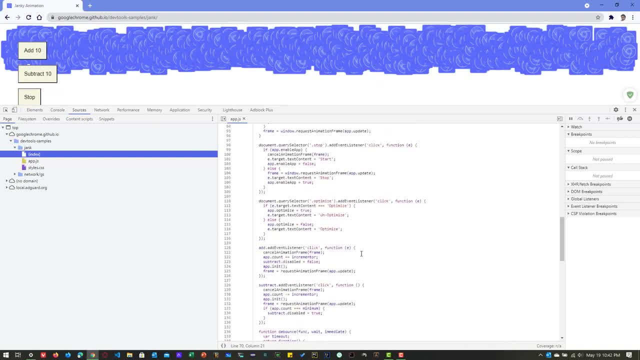 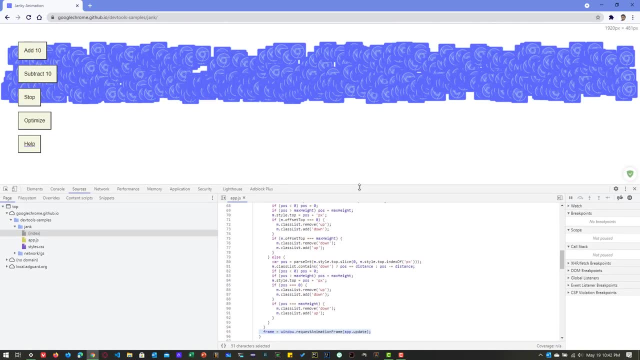 number which is causing the issue, and here the line number 90, 91 and so on. So these are the line you can optimize. So this particular app comes with the optimize button, basically. So now I'm going to click on this optimize. 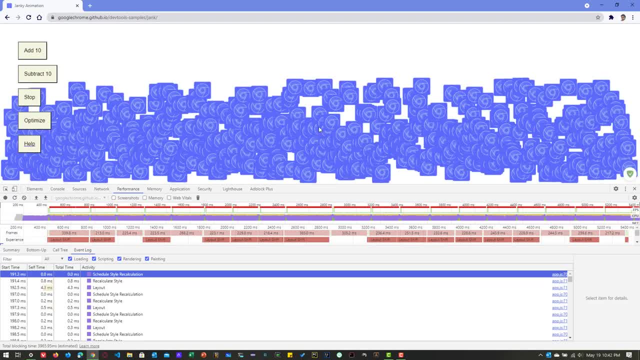 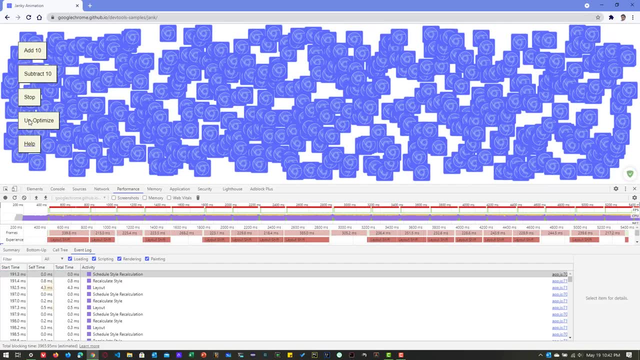 So once I click on this optimize, you can see these objects will move a little bit faster. So I'm going to click on this optimize. So now you can see it is moving faster and better than the previous settings. And if I click on unoptimized again, it will move slowly. 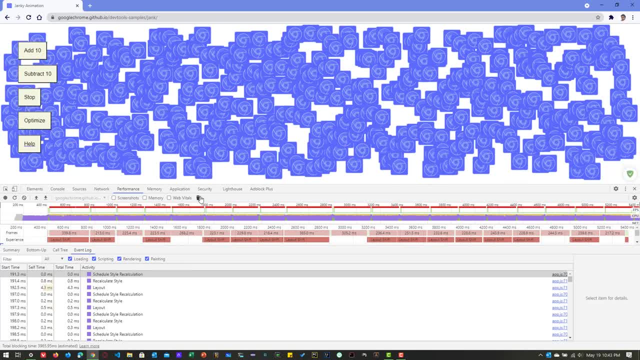 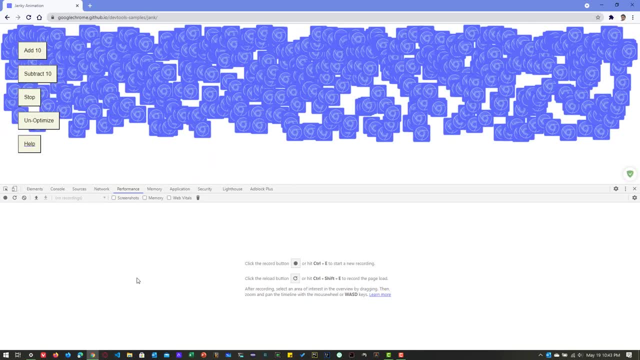 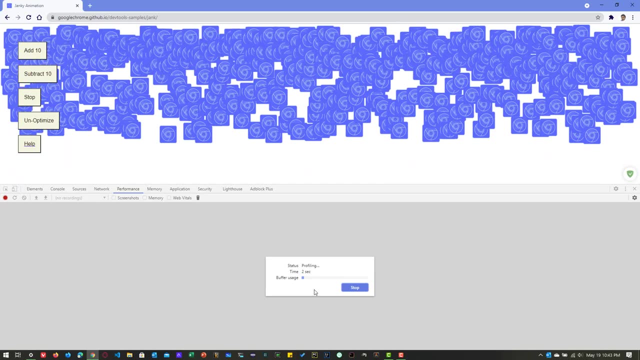 So now I'm going to clear this particular collection. So I'm going to clear everything and I'm going to click on optimize. So now the application performance is better and I'm going to take the snapshot again for about five seconds and I'm going to click on stop. 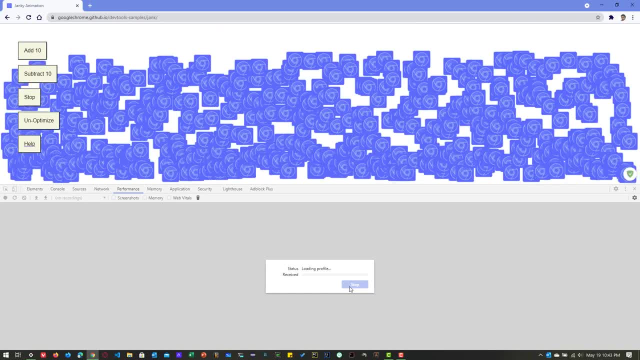 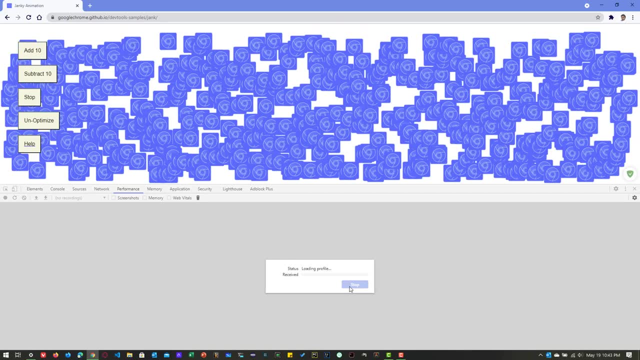 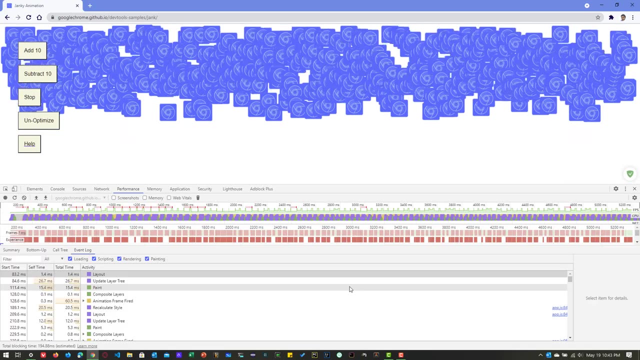 So now what will happen is you can see a lot of green colors instead of the red ones, And if you expand the main section in the information panel, you don't see much of a red color, basically. So now let us wait for a couple of seconds to see the details. 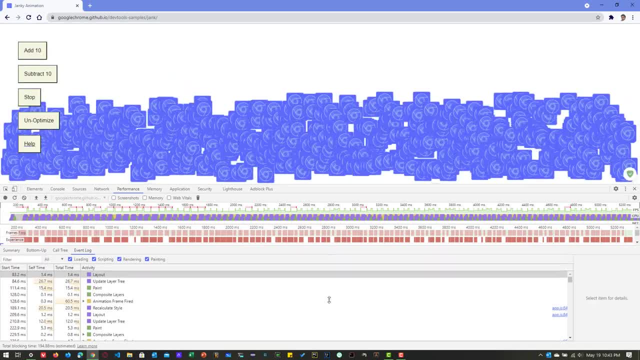 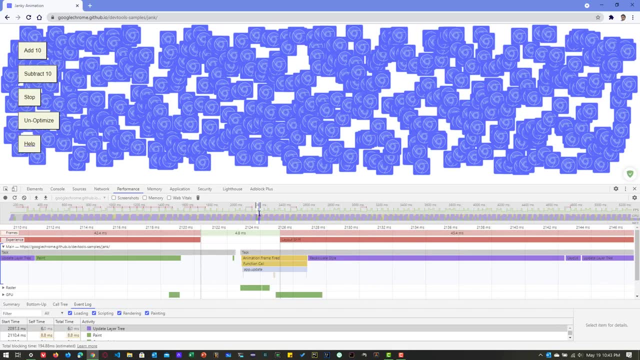 So now the profiling is done and here, if you just move this particular button here and you can see a lot of green ones, and compared to the red frames You can see there are a couple of red chunks we are seeing, but mostly we are seeing the. 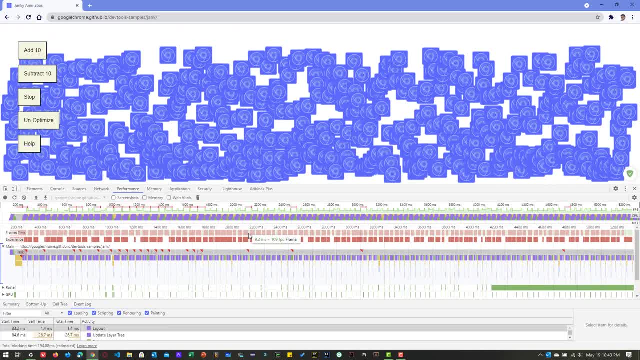 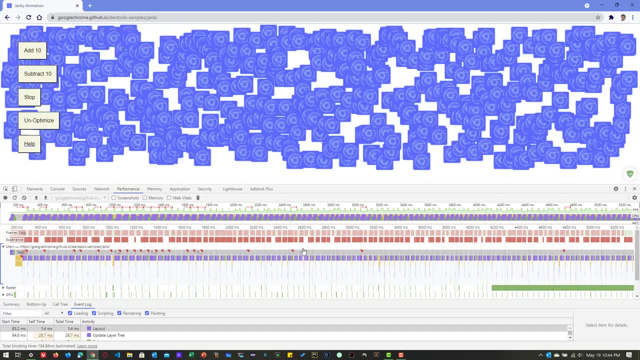 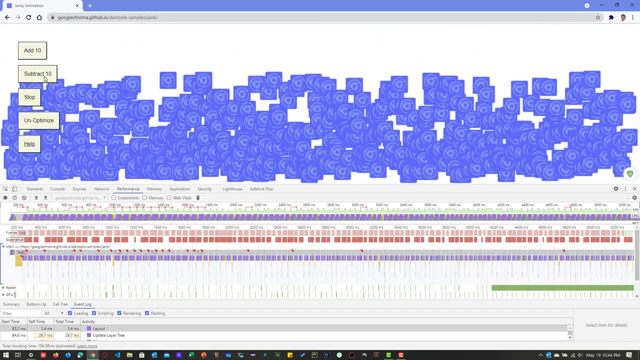 green ones And if you just move your mouse over you can see the information again. There is still. there is a long task, but it is previously better than the earlier version. And if you reduce the number of blocks again, you don't see the red color chunks here. 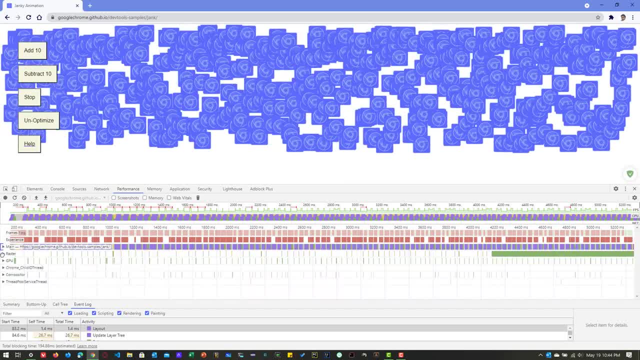 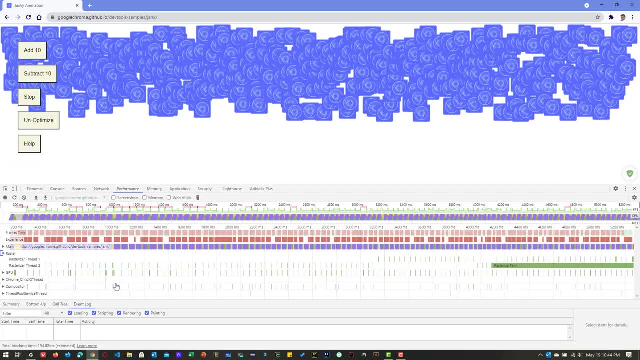 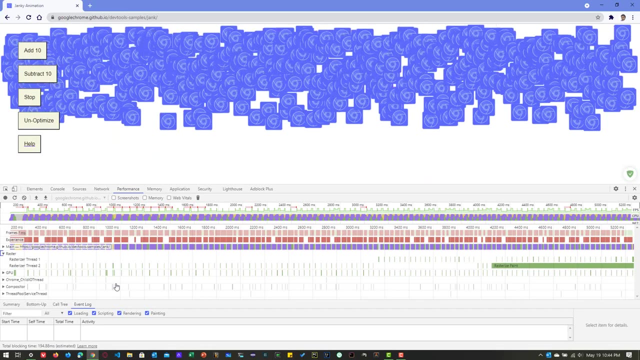 And here again, if you just close this main and if you expand the raster And if you expand the GPU, Chrome compositor, so you can see all the details. So these bottleneck analysis needs more knowledge about these terms. So I'm just trying to explain how you can get started with the performance bottleneck. 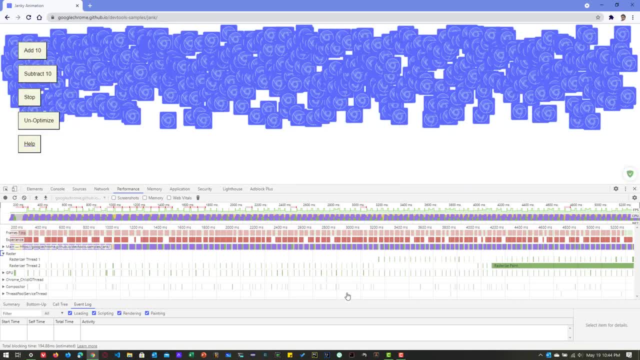 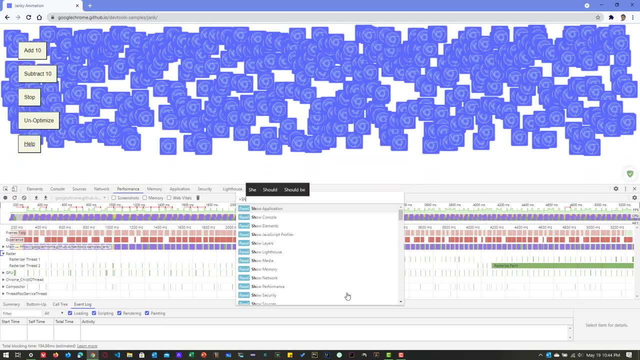 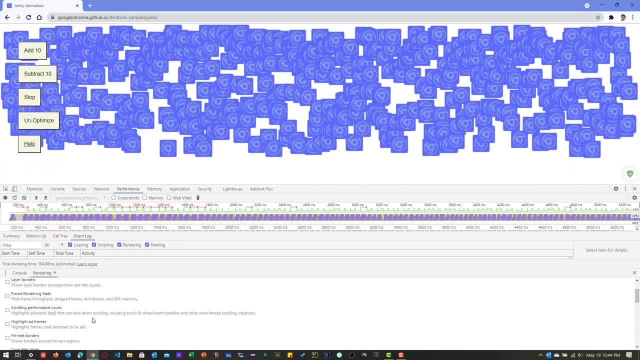 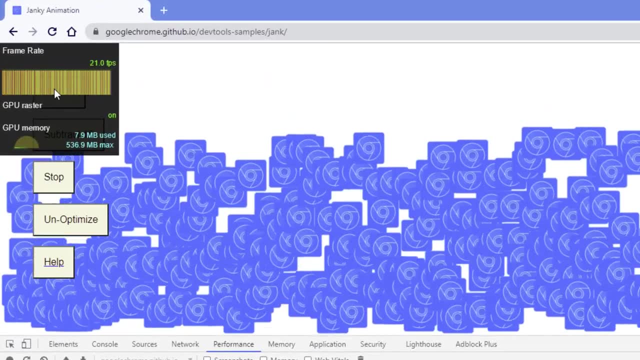 So this will bring up this, And here, if you just scroll down, you can see there is one utility called frame rendering stats. So if you check this box at the bottom you will get the frame rendering that utility- small utility- And here you can see a lot of greens and small chunk of reds, just going on. 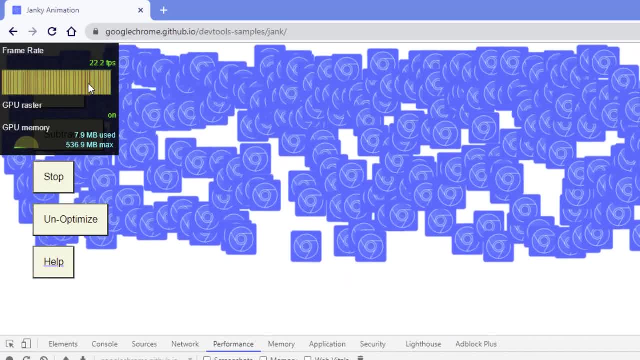 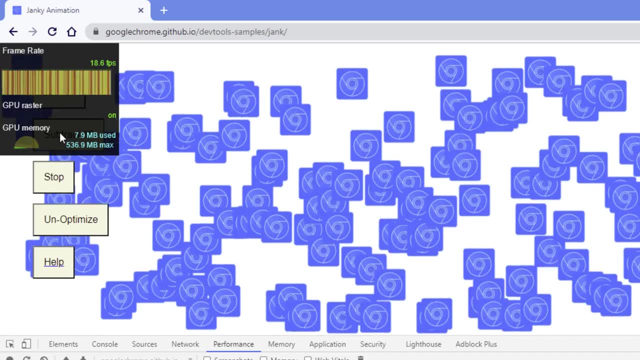 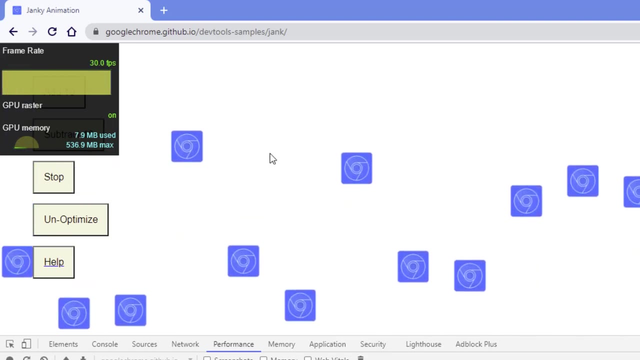 So this is the frames per second. So 60 frames per second means it is a decent frames and I'm going to reduce the blocks so that you can clearly see the green ones. So here, if you see a lot of green ones and if you keep reducing the images, you can see. 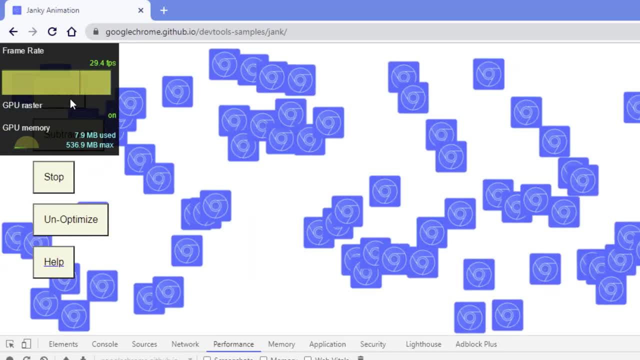 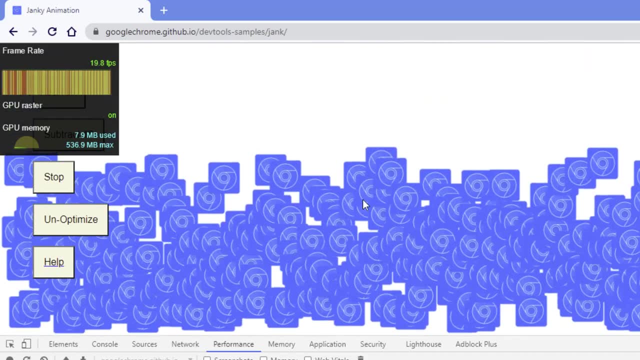 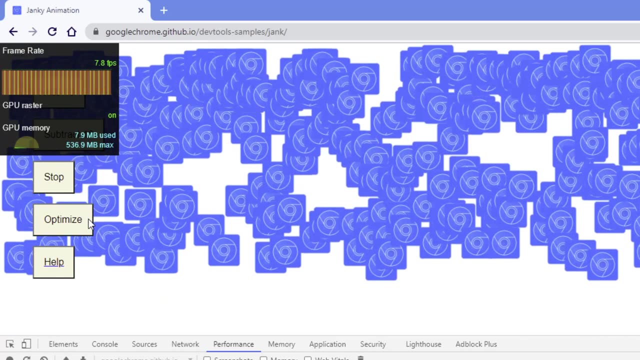 everything is green. Now if I click on again, add the images again and keep clicking, then you will see a lot of red chunks, and if I click on unoptimized again, you will see increase in the red chunks. So that is the whole idea of this demo application. 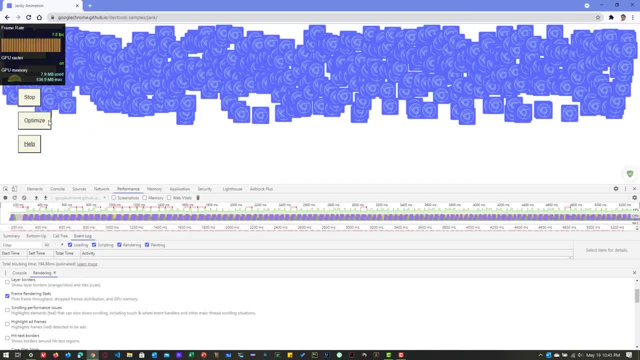 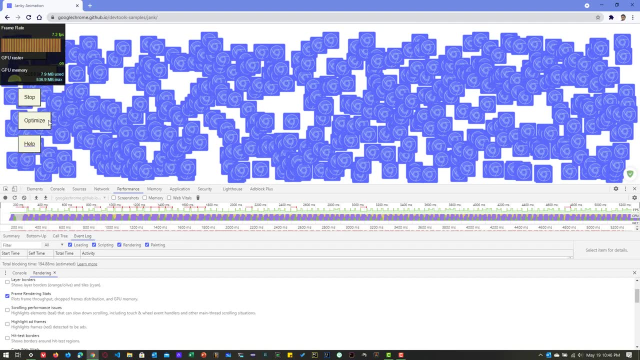 So this is how you get started with your analysis: using the performance tab, and then you will analyze what's going on by hovering your mouse over the pie chart and the frame chart. Then you can pinpoint the line number and then you can take the meaningful action. 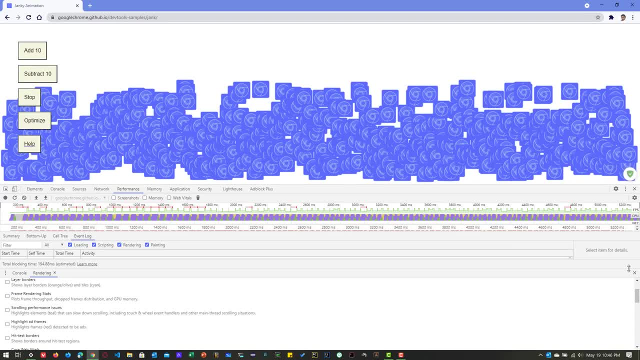 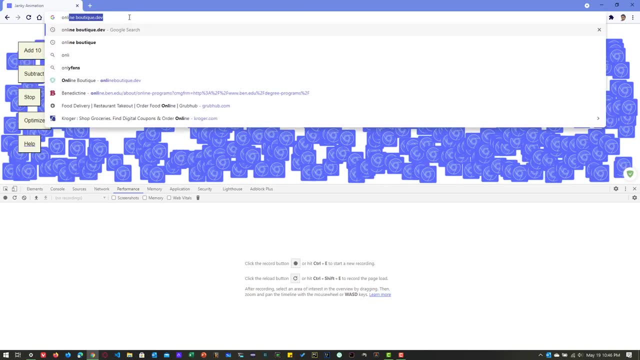 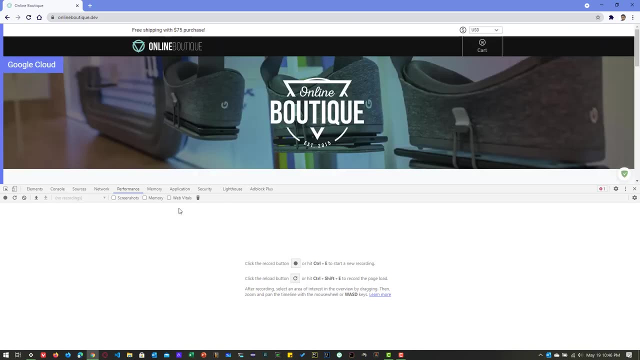 So, before I leave again, I want to tell you another important thing, which is web vitals. So I'm going to clear this and let us go to the online boutiquedev. So there's another sample website from Google and here I'm going to check this box: web vitals. 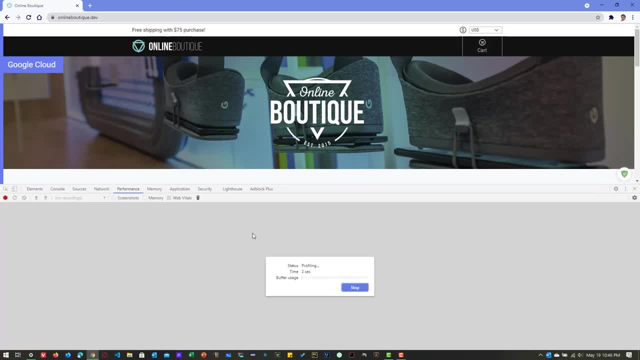 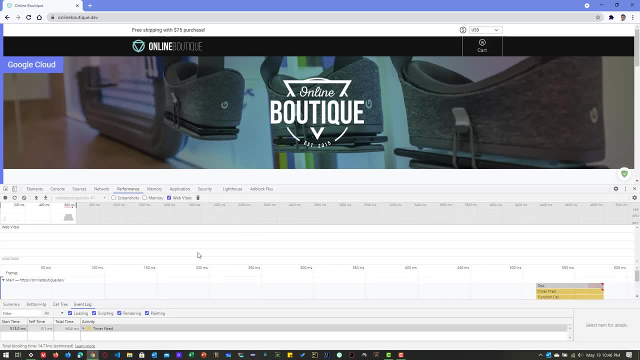 and I'm going to profile this particular website. Let us wait for three to five seconds and then click on stop. So this web vitals will display the web vitals such as LCP, LS, So those four categories it will display. So here I'm not seeing anything. 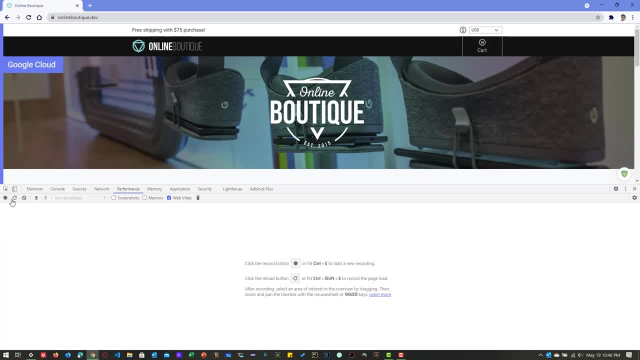 So what I can do is I can just remove this And I'm going to Hit record and I'm going to refresh this page Now. I'm going to stop. I hope now the web vitals should display, and yes, it is displaying. 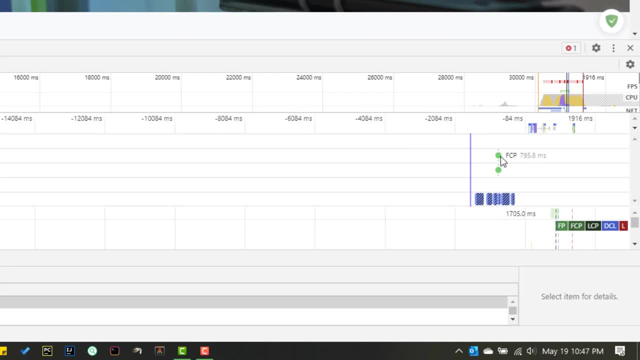 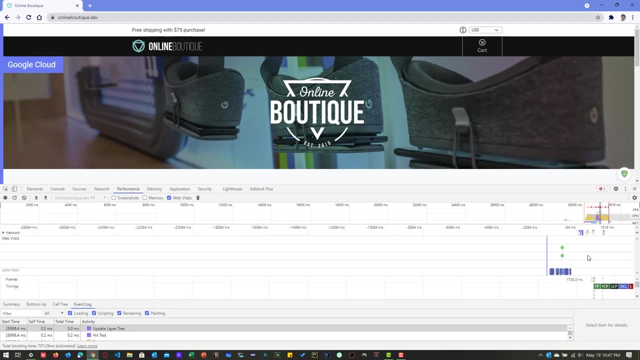 So now you can see here under the web vitals section, you can see the FCP and the first contentful paint and LCP, largest contentful paint. So everything is in green, which means your application is working perfectly. So now what we can do, just to see the details. 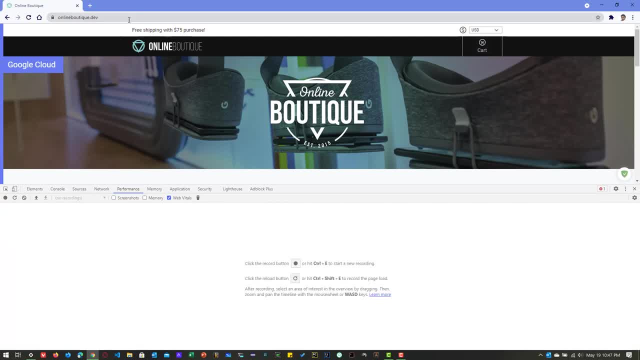 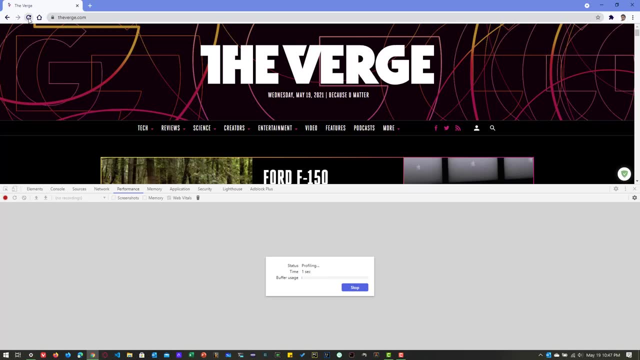 I'm going to delete this and I'm going to launch, say, the verge dot com and I'm going to capture this and I'm going to hit refresh again and let us hard refresh and stop So definitely. you can see some more information about the web vitals for this particular website. 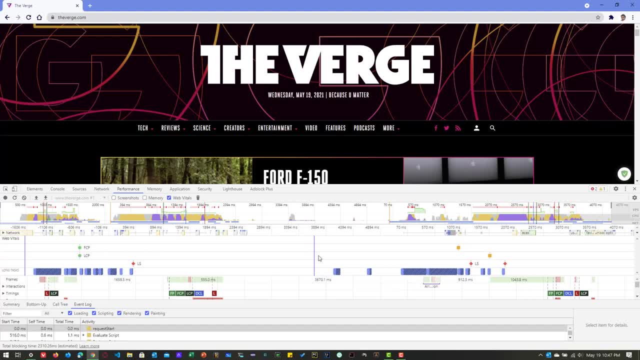 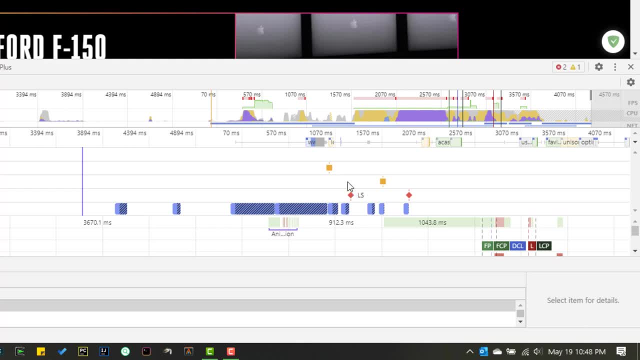 So here you can see FCP and LCP is good, But after the reducing the cache, removing the cache and hard reload, you can see there is a increase in the layout shift and first contentful paint and we can see again LCP and LS. 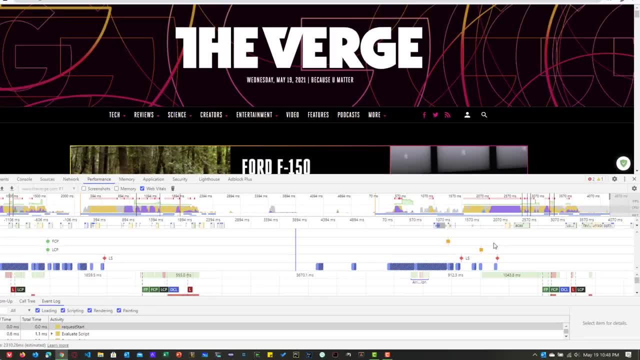 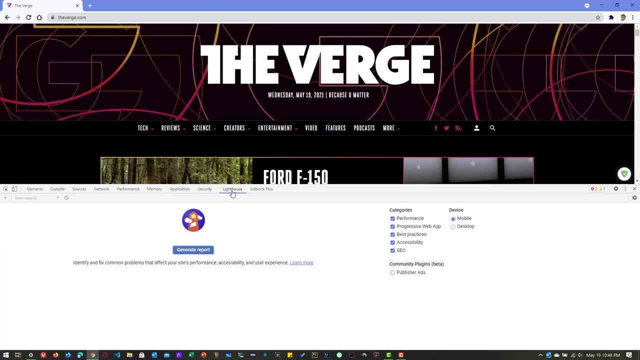 So you can see all your web vitals from this panel as well. But if you want to drill down into more details, you can use the lighthouse, which we are going to see in next video, And also you can leverage the web dot dev. 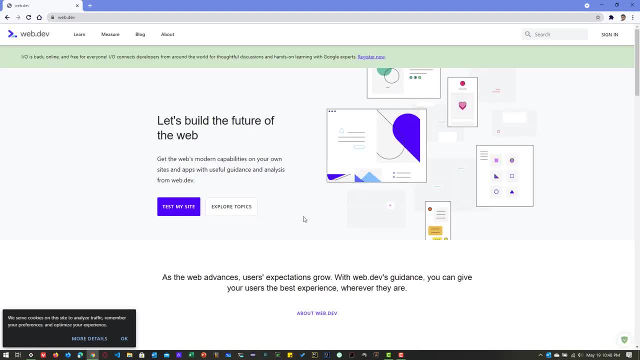 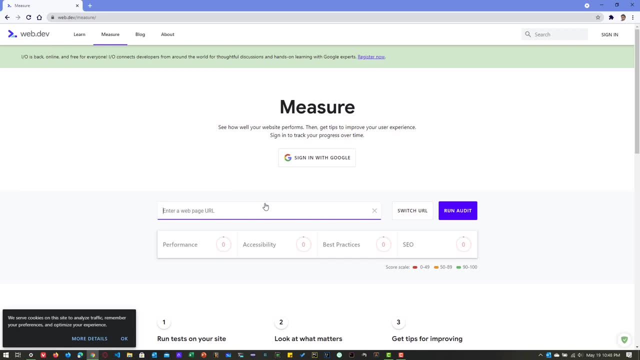 So this is another A website where you can measure your website performance by clicking on this test my site button and feed your URL to run the audit, So which also we are going to see in the next couple of videos. So I hope this video will help you to get started with the performance bottleneck analysis. 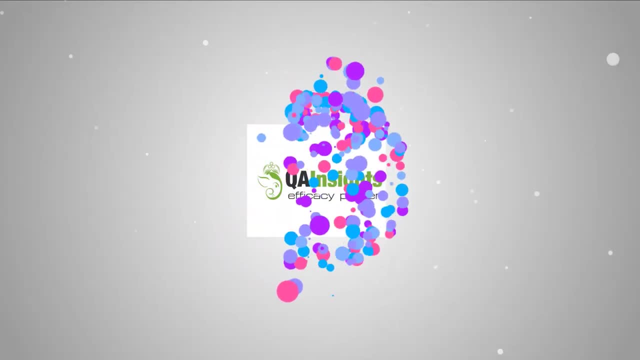 and thanks for watching. Have a good day. If you like my dad's videos, please subscribe to QA insights channel.